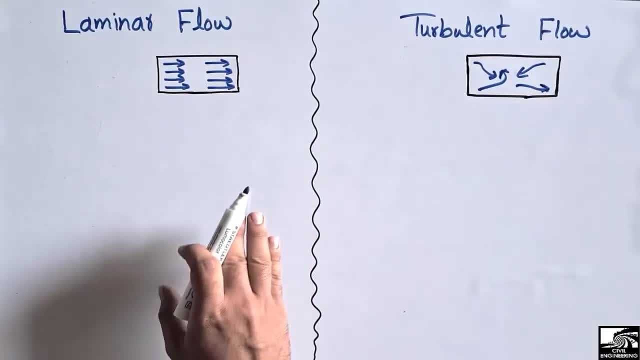 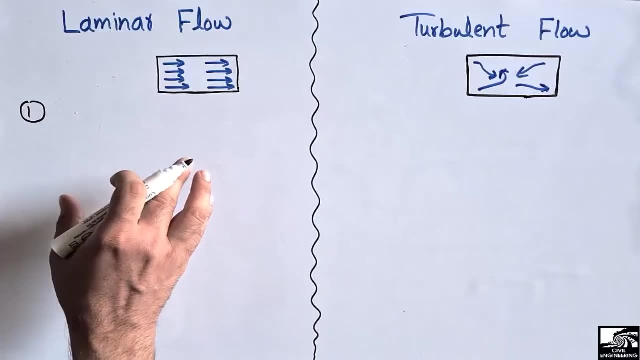 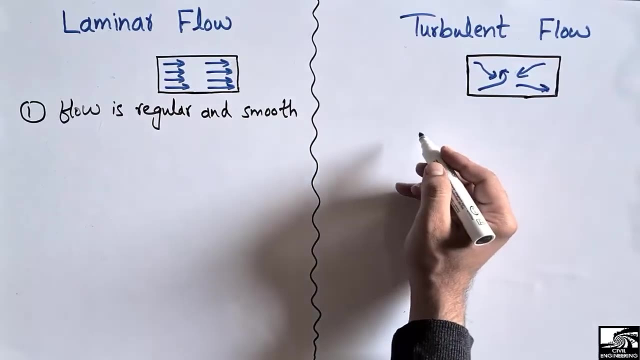 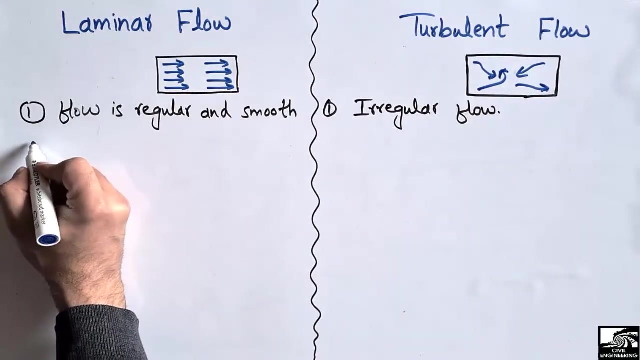 flow. But there are also some other characteristics of these types of flow. For example, if we look at the flow of the fluid, we can see that the flow of the fluid is regular and smooth, while the turbulent flow is irregular. The second characteristic of the laminar flow. 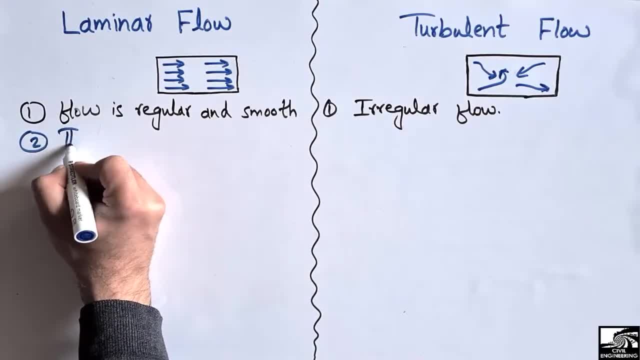 is that the value of the Reynolds number is less than 2000.. So the value of the Reynolds number is less than 2000.. So we can see here that the flow is irregular and smooth, while the turbulent flow is irregular. So such type of flow is called as the turbulent flow. For 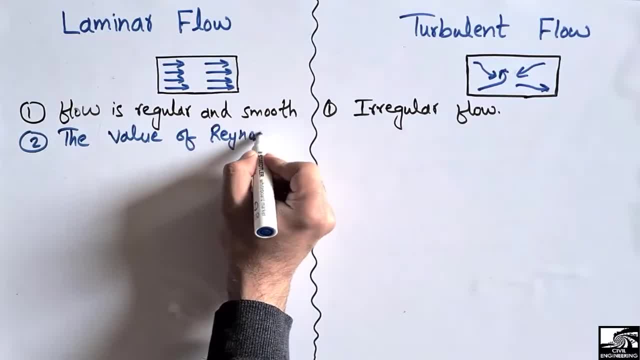 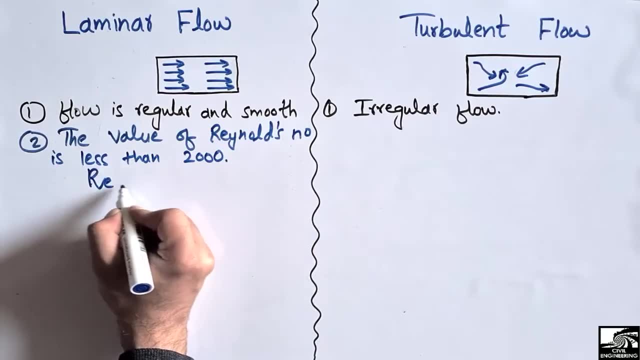 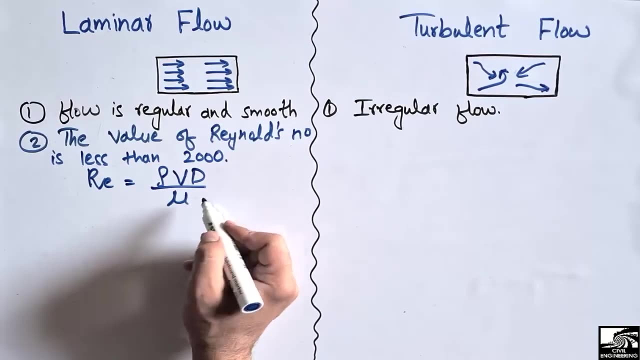 example, if we look at the flow of the fluid, we can see that the flow of the fluid is less than 2000.. And the Reynolds number is represented here by re, which is equal to rho of V divided by mu. So for the case of the laminar flow, the value of the Reynolds number should be: 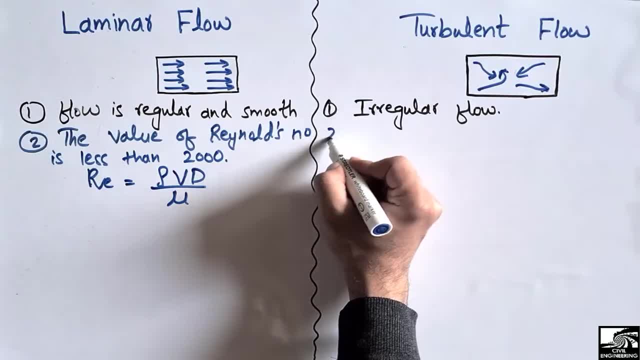 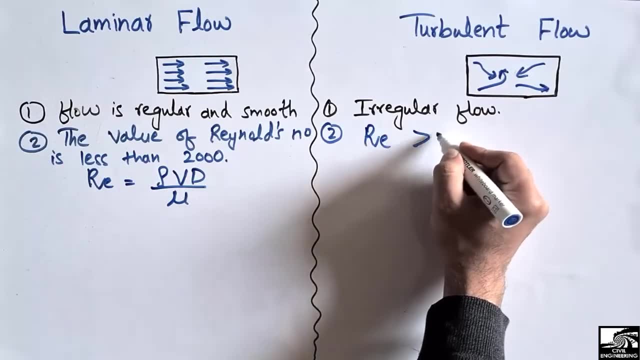 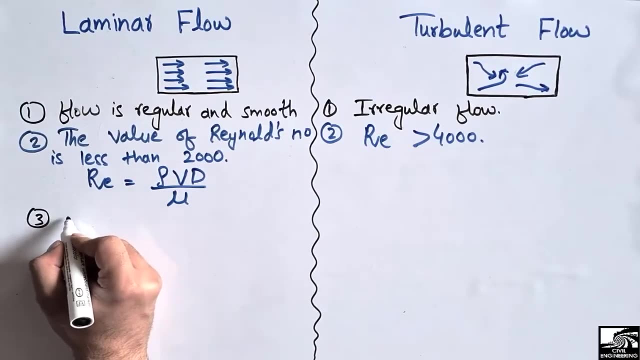 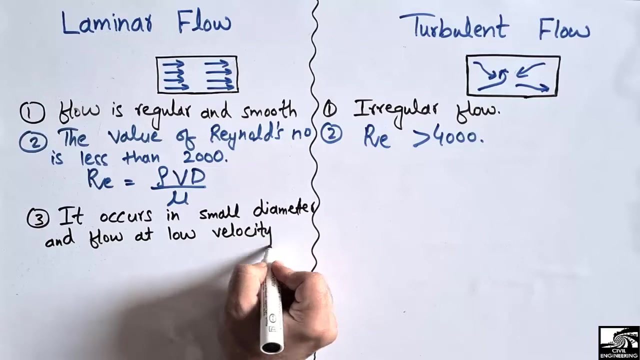 less than 2000,. while for the turbulent flow, the Reynolds number value should always be greater than 4000.. The third characteristic is so: the third characteristic for the liminal flow is that it occurs in smaller diameter of pipe and flow at low velocity. 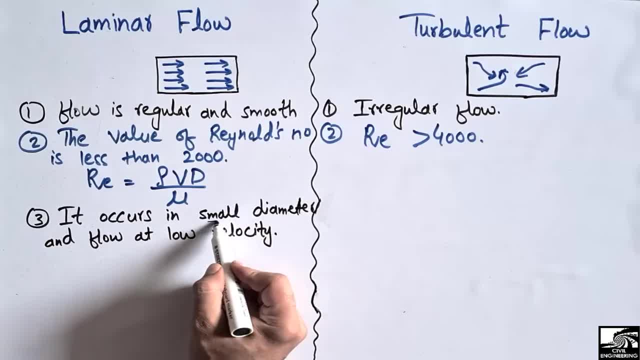 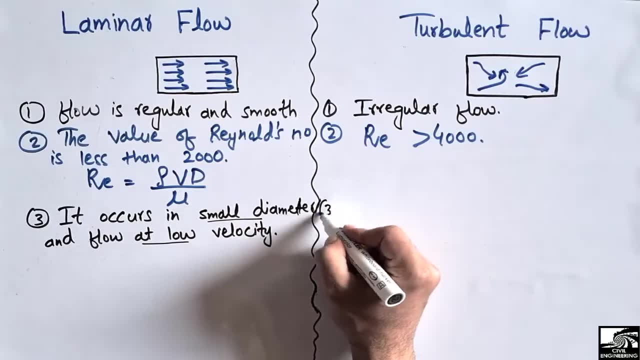 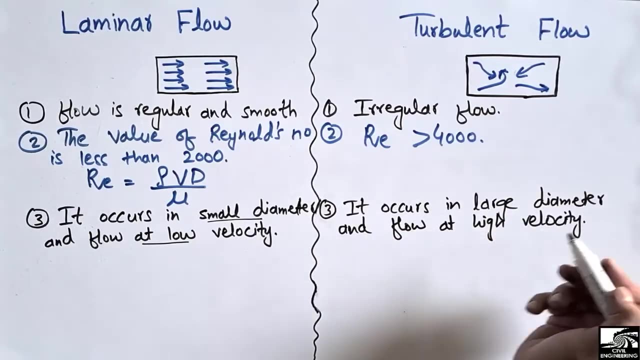 So this will be the liminal flow if it occurs in the smaller diameter of pipe and always flow at a low velocity. so we will have the liminal flow while for the turbulent flow. so for the turbulent flow it mostly occurs in the larger diameter of pipe and it flows. 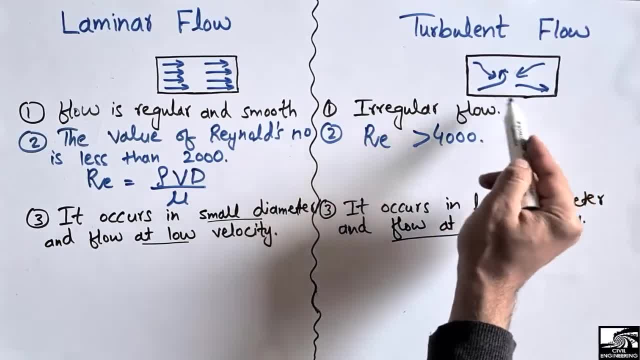 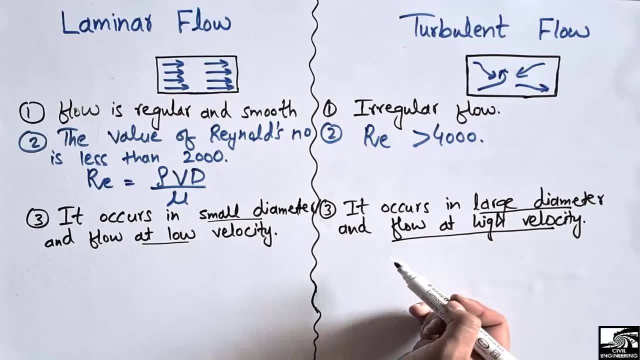 at a high velocity So we have more disturbance. so when we have more disturbance in our flow, we call it the turbulent flow. So this was the third characteristic of these two types of the flow. And the fourth characteristic of the liminal flow is that all the fluid layers of the liminal 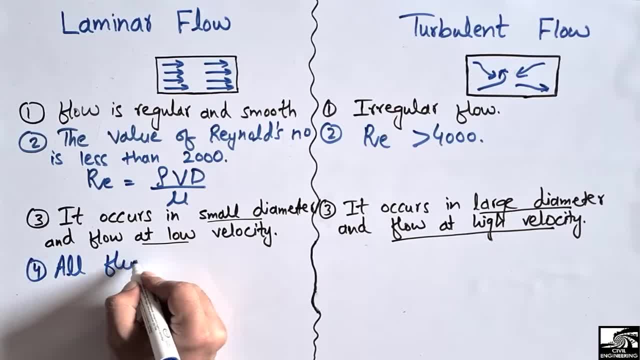 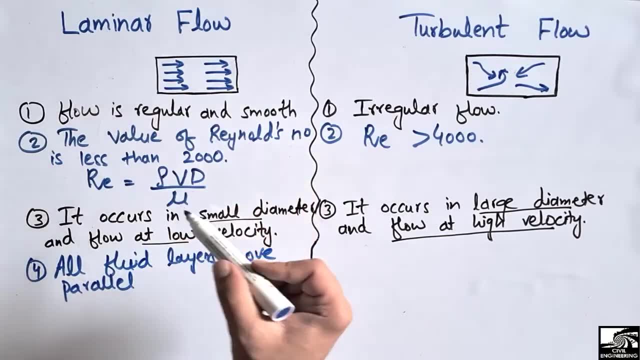 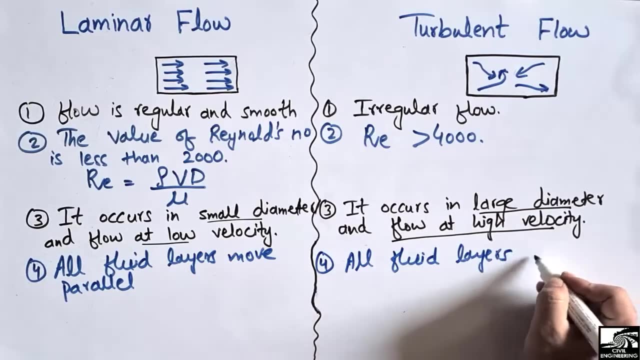 flow move parallel. So all the fluid layers move parallel in case of the liminal flow, while in case of the turbulent flow, the all fluid layers do not move parallel. So in case of the turbulent flow, all the fluid layers should not be move parallel.